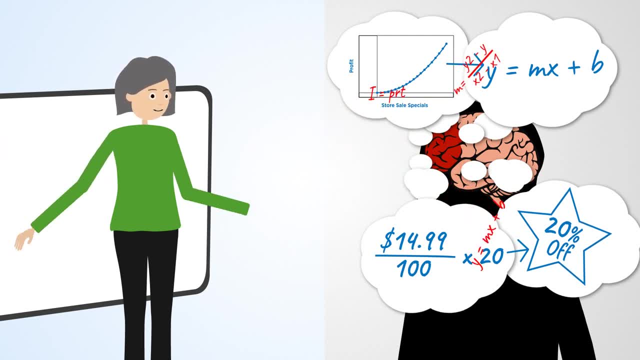 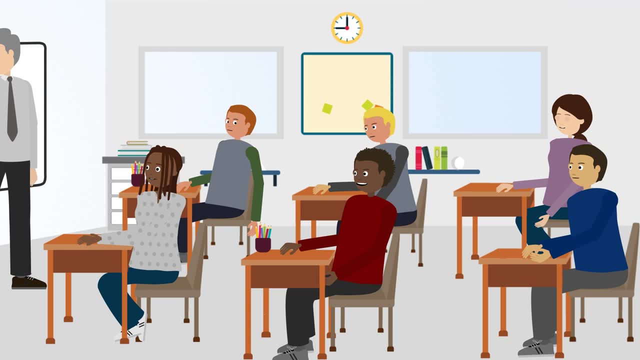 which increases what psychologists call cognitive load. This can block cognitive flexibility and prevent adolescents from making important mathematical connections. His research revealed that math teachers who emphasize the connections between mathematical concepts and consistently improve their cognitive ability, and they can also improve their cognitive ability. 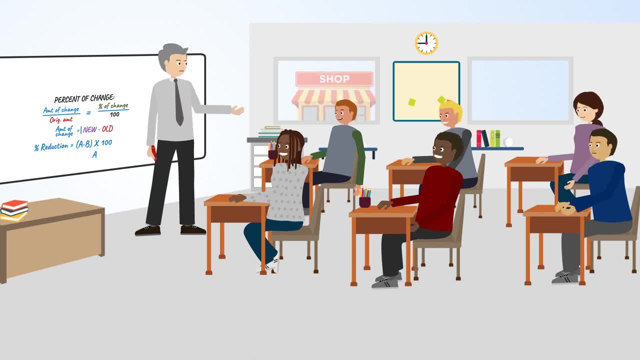 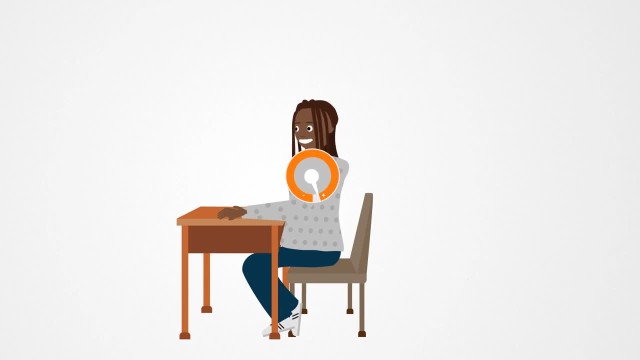 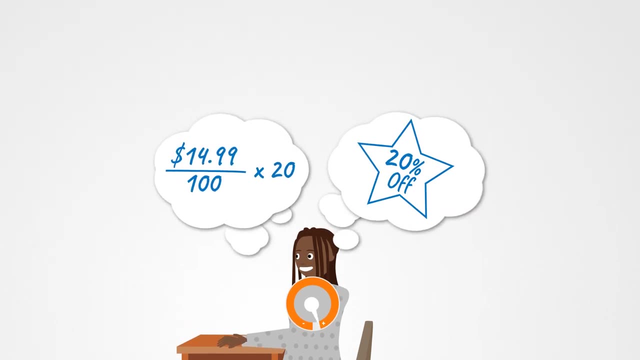 by providing concrete real-world examples, increase students' internalized value of math. These students did not just become more interested in math, they were beginning to build an identity around math. Dr Matthews also found that TMAs and cognitive flexibility work together to predict students' value of math. 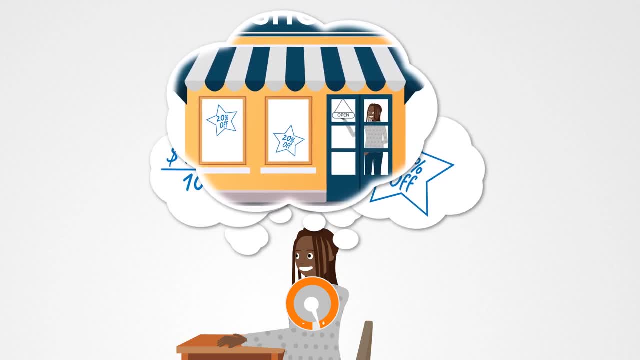 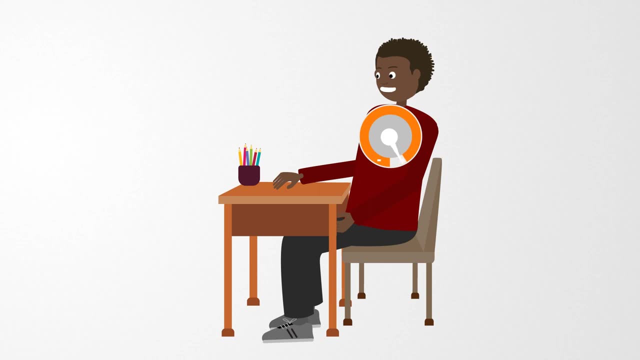 Greater maturation and cognitive flexibility help adolescents process and internalize TMAs for their own sense of math identity. Those in math classrooms and those in classrooms with less TMAs were more likely to express frustration, uncertainty and a negative opinion of math. 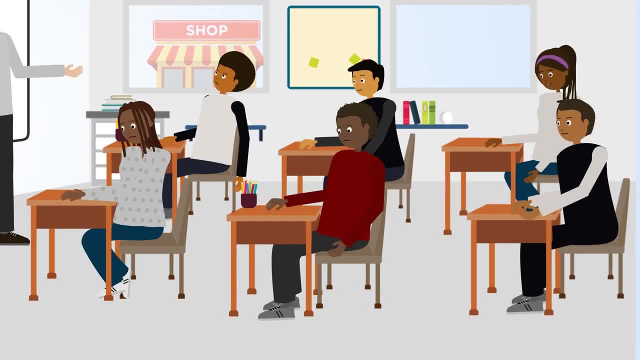 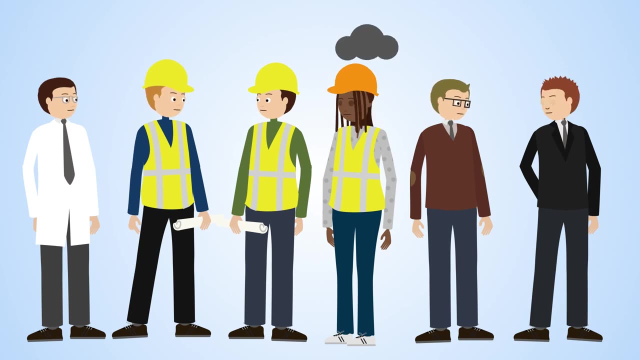 But there's more: Black, Latino and economically disadvantaged adolescents often face additional challenges like racial stigma and stereotypes that can make it even more difficult for them to realize the value of math for their lives. These students are also typically underrepresented in math-related degrees and careers. 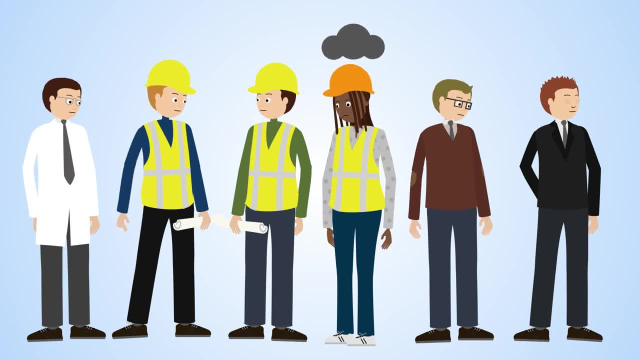 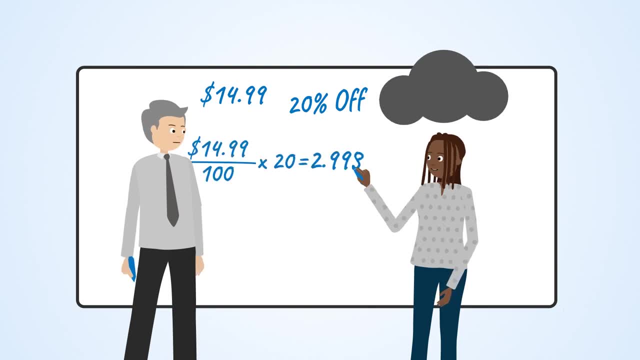 which can reinforce stigma or a lack of belonging, Dr Matthews said. Dr Matthews followed up on this by interviewing students one-on-one to understand their beliefs about race and how they experienced and managed stigma. in math, He found that, while some students struggle with stereotypes, 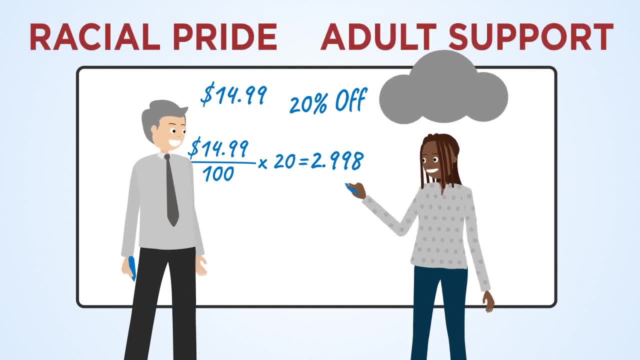 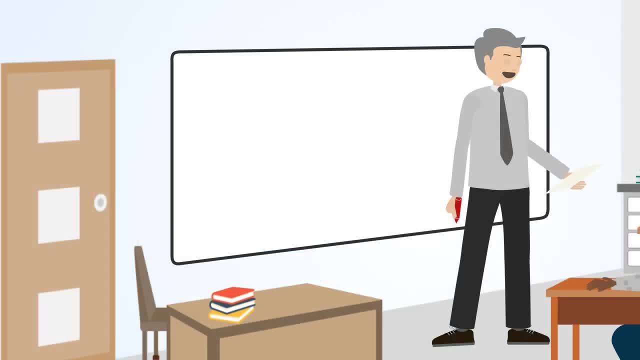 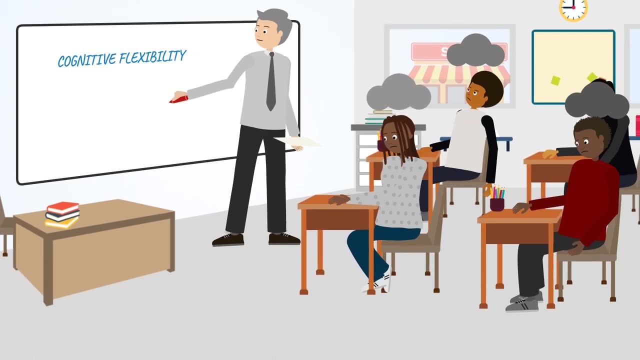 other students with racial pride and adult support saw achieving success in math as an opportunity to resist stigma and prove doubters wrong. Dr Matthews has begun to turnkey his findings into developing practical tips for teachers. Some of these strategies include how to understand and support cognitive flexibility. 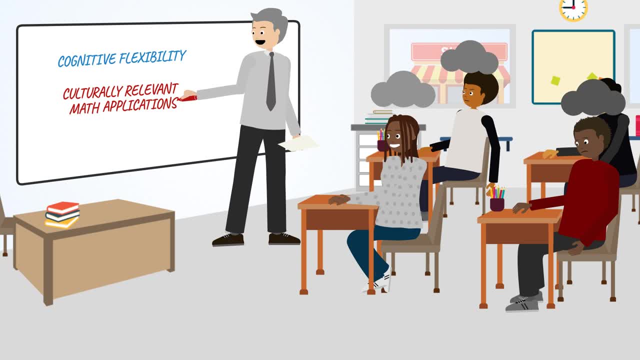 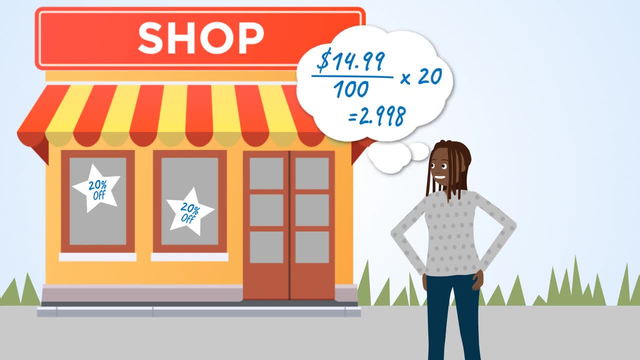 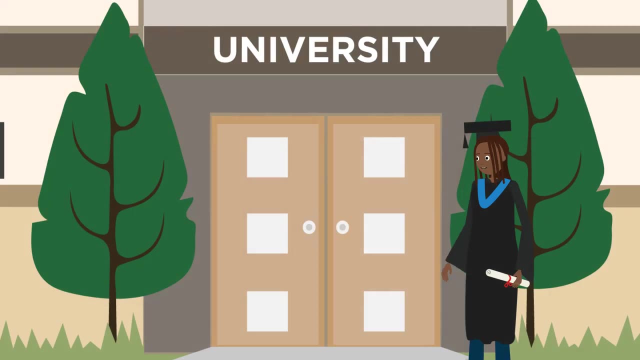 or how to develop culturally relevant math applications to reinforce that Black and Latino students do belong as mathematicians. By advocating a better understanding of students' interests and experiences, Dr Matthews' research empowers teachers to help students appreciate the value of math. This support can be instrumental in creating opportunities for access and equity in higher education and beyond. For more information, visit wwwfemaedu.